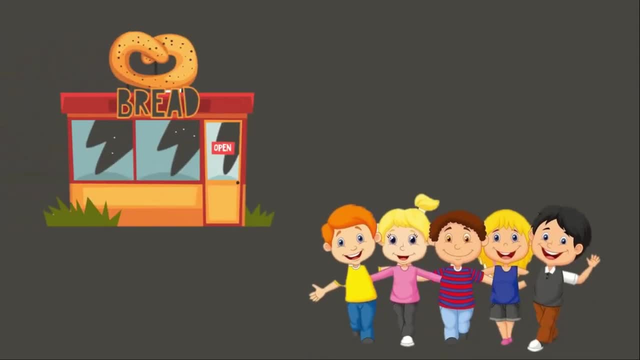 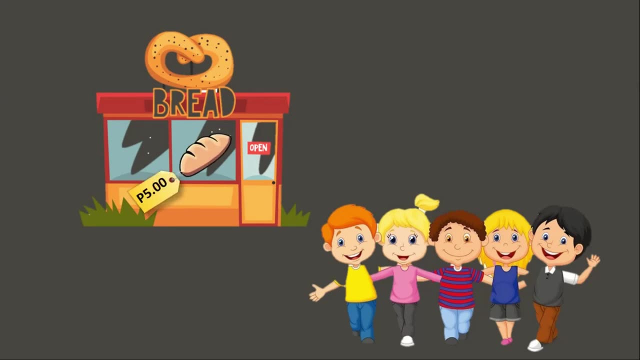 There are five kids who went to the bakery store to buy some breads. A piece of bread costs five pesos. If each one of them bought five breads, how much did they pay in all? Now, let's try to solve this one. Do you have any idea? 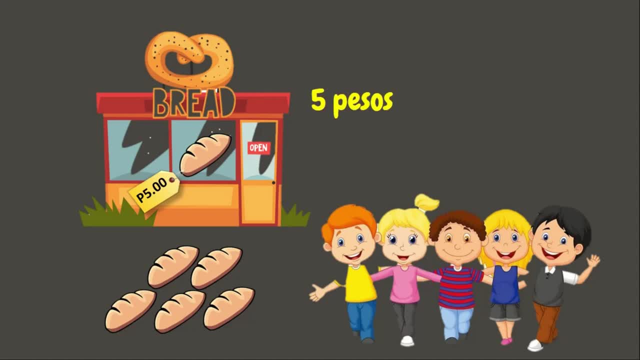 That is right. We need to multiply five pesos, which is the cost of the bread, to the number of bread each one of them bought, which is five bread, to the number of kids, which is five kids. This gives us our number sentence: five times five times five, which is one hundred twenty-five. 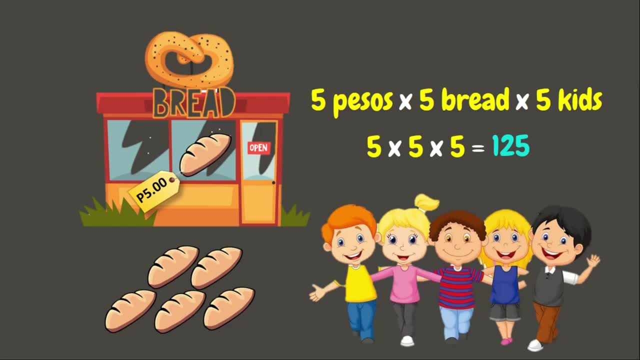 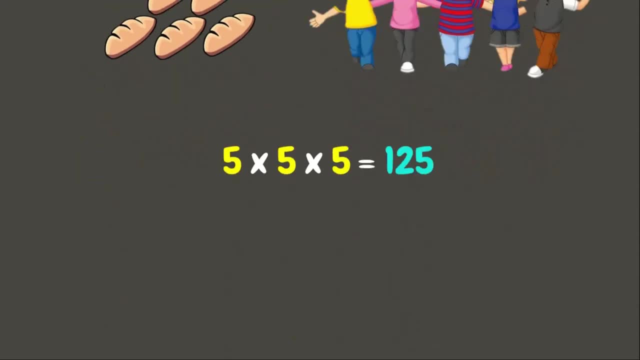 Very good. This means that they paid one hundred twenty-five pesos in all Wonderful. As you look at this equation, we can see that number five is multiplied repeatedly to the number of children who went to the bakery store to buy some breads. 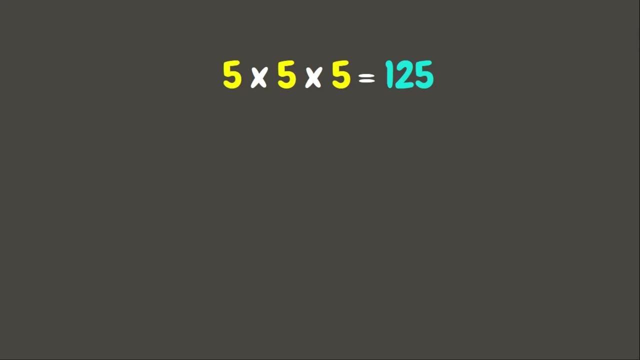 Let's try to solve this one. Do you have any idea? There are five kids who went to the bakery store to buy some breads. This equation can be also written in a different form, wherein five is multiplied repeatedly to itself three times. 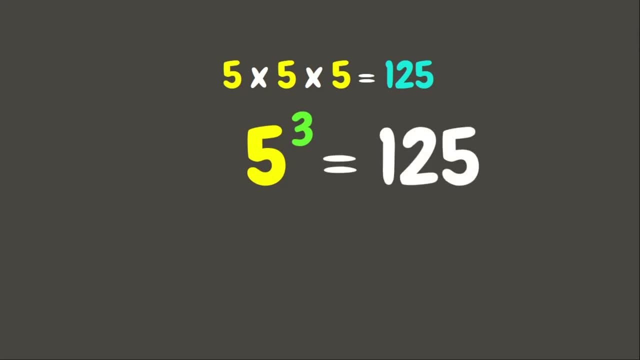 is equal one hundred twenty-five. This is an example of exponential form or exponential notation. Exponential notation is an example of exponential notation. form or exponential notation is another way of expressing numbers. it has two parts. the number that is being multiplied repeatedly is called the base. 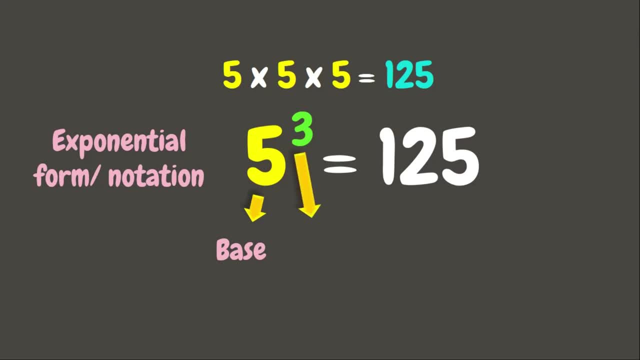 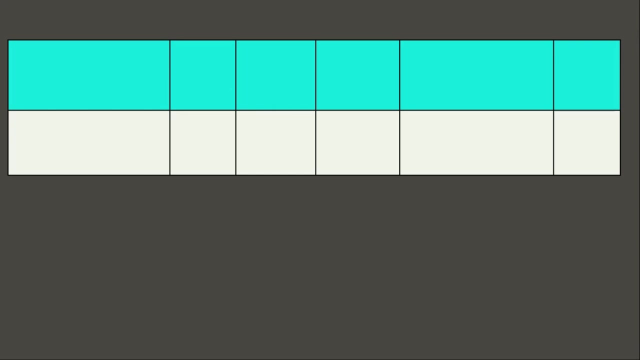 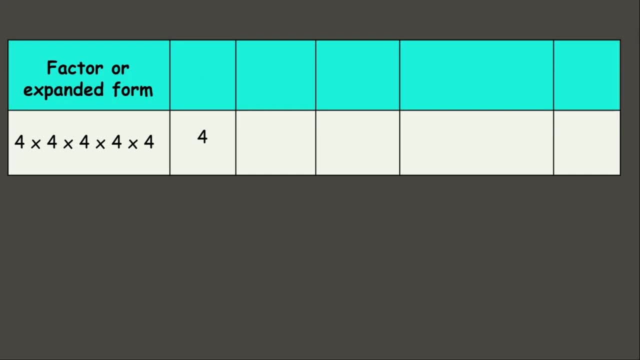 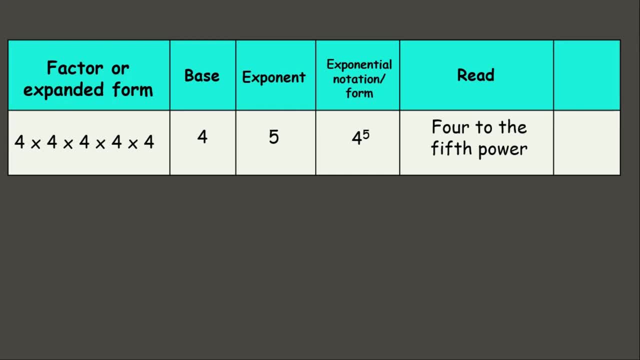 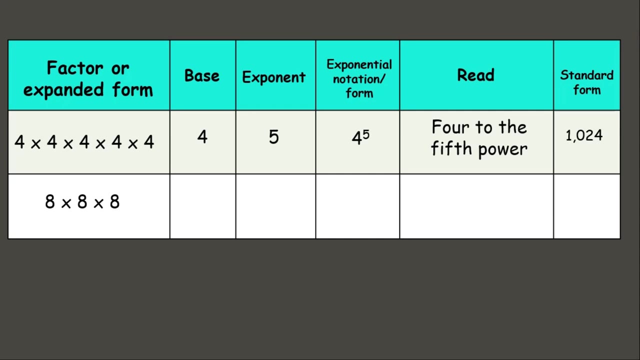 times four times four, that gives us 1024, and this is the standard form. now let's have another one. we have here 8 times 8 times 8, we can see that eight is being multiplied repeatedly. so that is our base, and the base is being multiplied three times. so 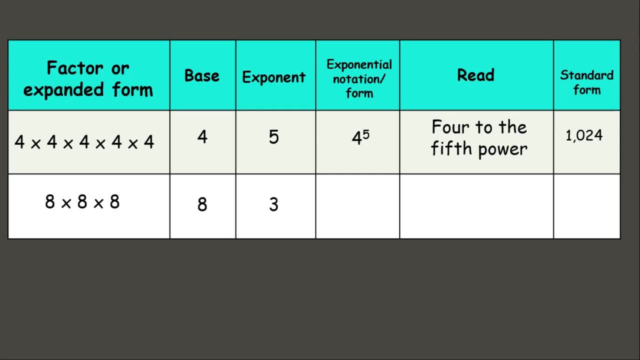 that is our plumlet, that is our equivalent, our exponent, when written in an exponential notation, that is, 8 to the third power, or 8 cube. when solved, this gives us the standard form, which is 8 times 8 times 8 equals 512. let's have another one. we have here 12 times. 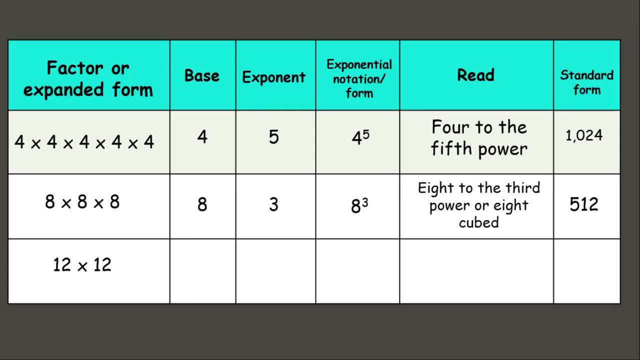 12. the base here is 12 and the base is being multiplied two times. so that is our exponent. now let us write down its exponential notation. there you go, and we can read this as: 12 to the second power, or 12 squared, which gives us the value. 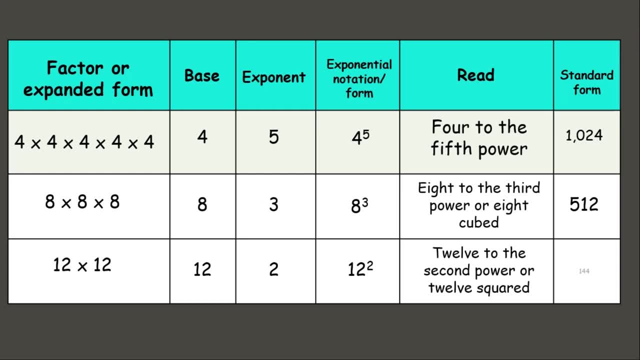 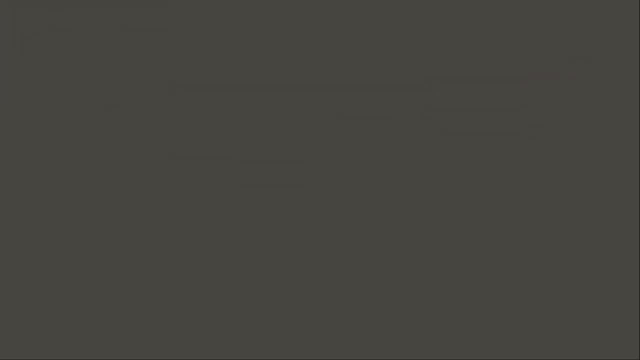 12 times 12 equals 144. wonderful, now let me give you some previous. did you know that all numbers have its invisible exponent? yes, all numbers have invisible exponent of 1. when a number has an exponent of 1, it is always equal to the number itself. so 5 raised to 1 is 5 to 1. 4 to the first power is 24 and 9. 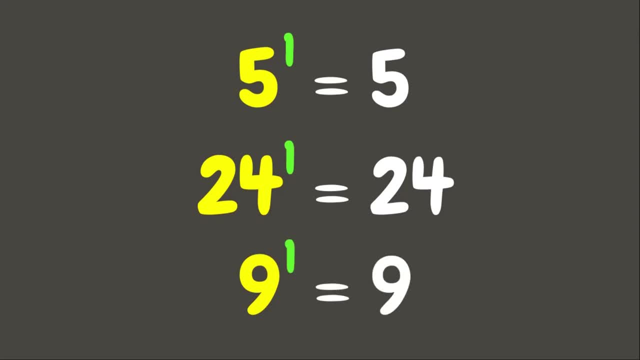 to the first. power is 9. there you go. now let's have another one. when the number has the exponent zero, it is always equals to 1. 3 has an exponent of 0 is equals 1, and 34 has exponent of 0 is equal 1. again, when a number has an exponent of 0, its value is: 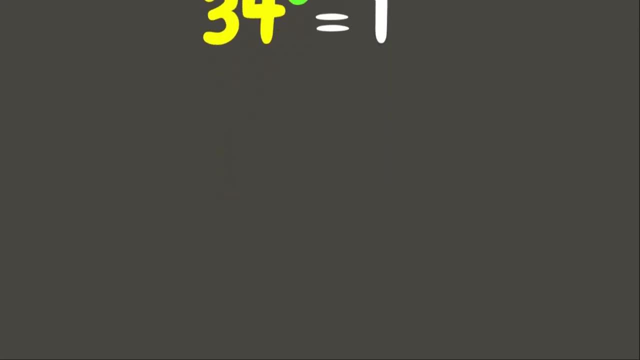 1. now let us try this one. I want you to look and observe: 10 has the exponent of 2 or 10. to the second power: when written in expanded form is 10 times 10 and when solved that gives us the value 100. then to the third power. 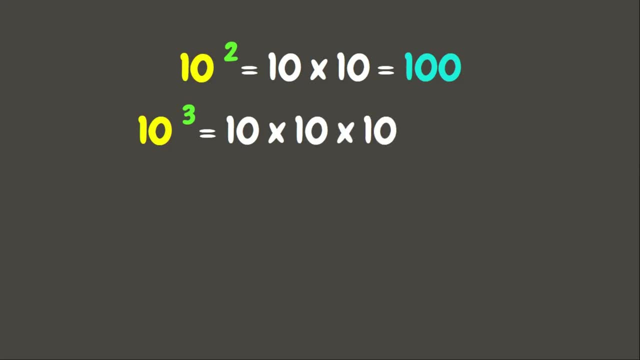 is 10 times 10 times 10, which is equal 1000, while 10 to the fourth power has the value of 10,000. and, lastly, 10 to the fifth power has the value of 100,000. now, as you can see, 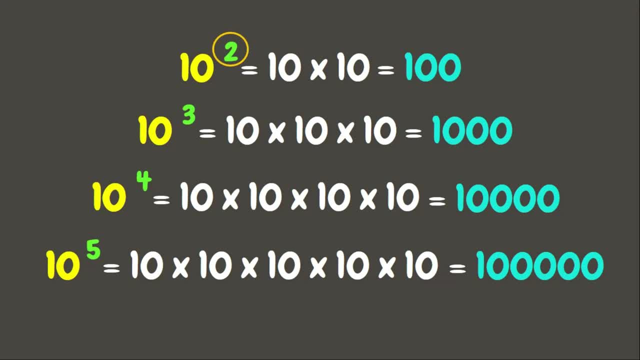 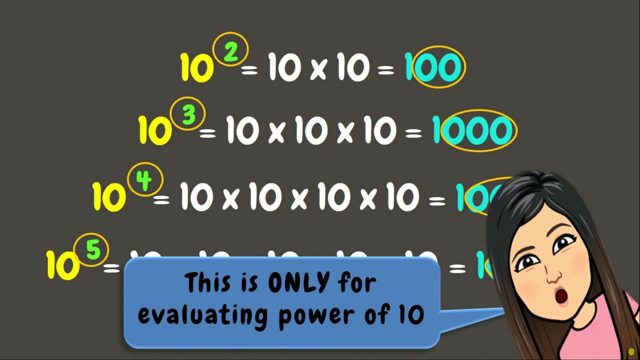 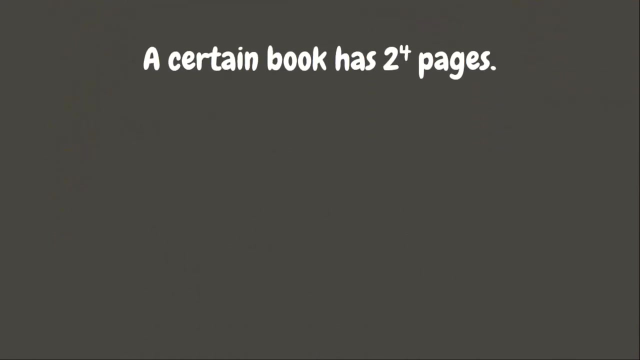 the exponent is the same as the number of zeros in its standard form. these are examples of power of 10. remember this is only for evaluating power of 10. wonderful examples is the form: about 100 million in total, now 50,000 and 50,000 vitesse is. 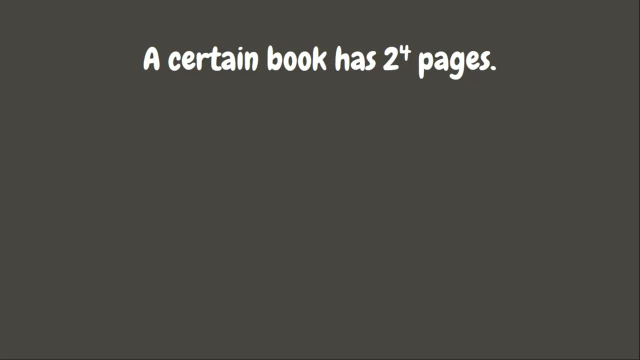 about 200 million how many wages does this super何 now a diameter of 200 틈 is equal 10 to the fourth самых emotions that we sort out by taking plus 30 thousand times 207 plus 20ule �� how many pages does this book have now how many pages does this book have now let us 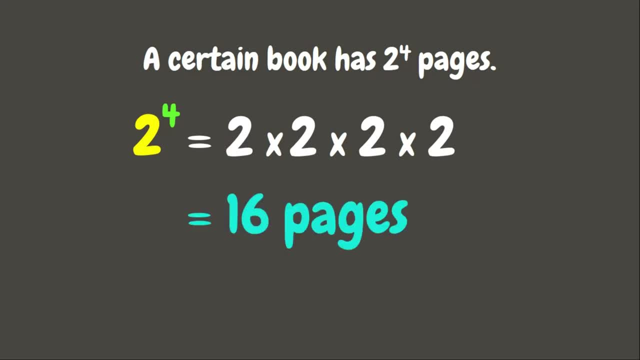 for this one that gives us 16. therefore, this book has 16 pages. wonderful. how about this one? what is seven to the fifth power? first, let's write it down in its exponential notation. we all know that the base here is the seven and exponent is the fifth power, which is five. now let's try to. 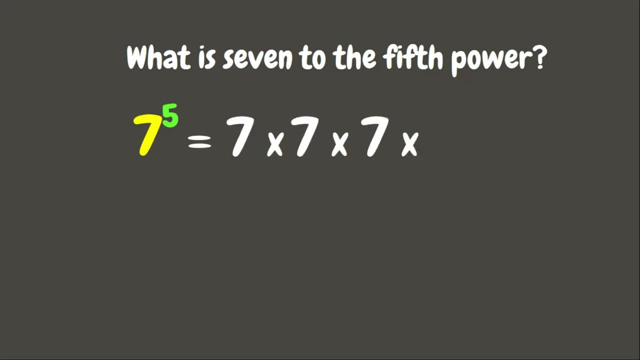